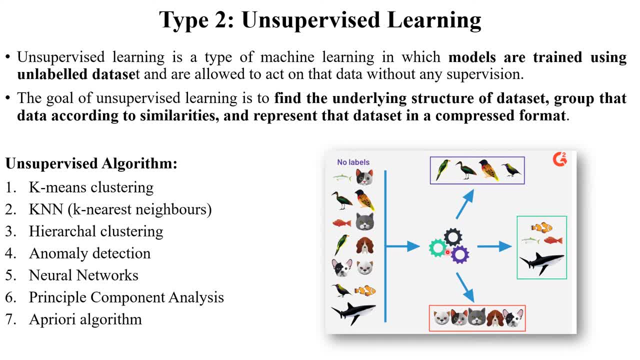 machine for the training purpose. So in unsupervised algorithm machine can be identify the structure of data set. Machine can identify the particular groups than particular functionality, similarities, than particular characteristics, structure of each and every animals. This, all things can be identified, the machine 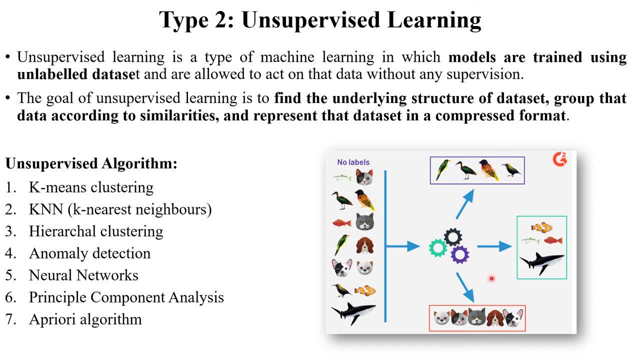 Then, after that day, can predict a particular result. So this is the concept of unsupervised learning algorithm. We didn't pass label data to the machine for training purpose, okay. So for that purpose we will use different algorithms like k-means, clustering, k-nearest. 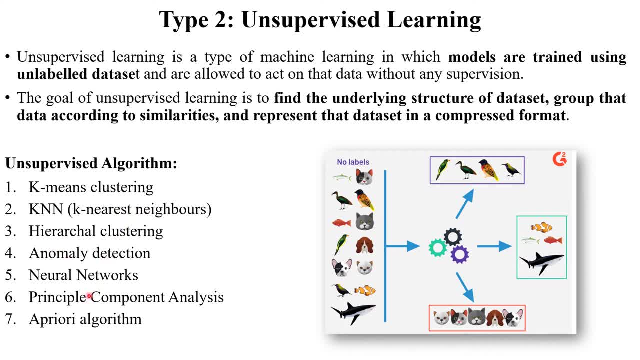 neighbor, hierarchical clustering, anomaly detection, neural networks, Principal component analysis and apriori algorithm. So we will learn all those algorithm in the next session. unsupervised learning algorithm is we will pass unlabeled data to the machine for training purpose and machine identify from those images and cluster them or group them as per their 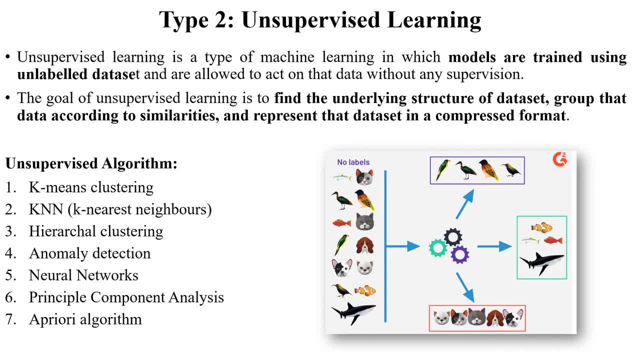 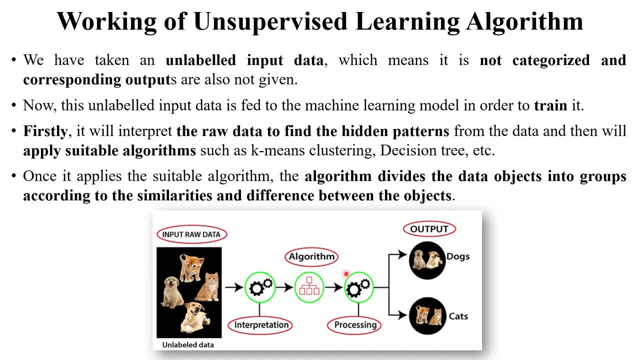 characteristics. this is a concept of unsupervised learning algorithm. next now see here: this is just working of unsupervised learning algorithm. in this image, see, in this image, there is a. there are total four images of. there are two images for cat and two images for dog. right, we will pass. 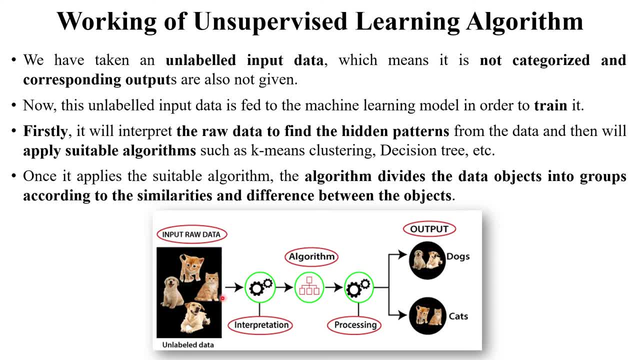 these images as a input to the machine. these are the unlabeled input data. there are only images right. this unlabeled input data pass to the machine for the training purpose. now machine can, by using some algorithms like k-means, clustering algorithm, decision tree algorithm, machine can be identify some pattern of that particular images. structure characteristics. 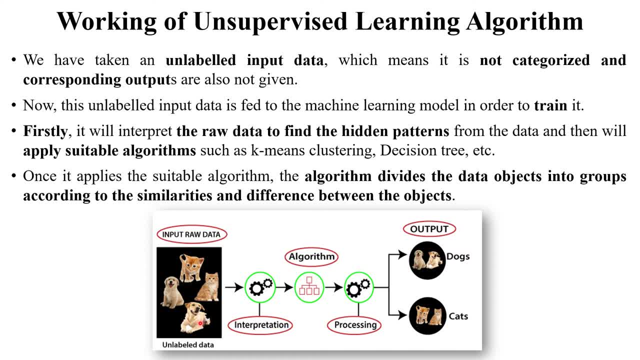 and right this. all kinds of specifications identify the machine for that particular images. okay, then, after training and after identifying the machine, the particular model can be generated, the particular groups of that data set. for example, see here there is a dogs and there are the kites. this is the output of that particular machine by using unsupervised learning algorithm. 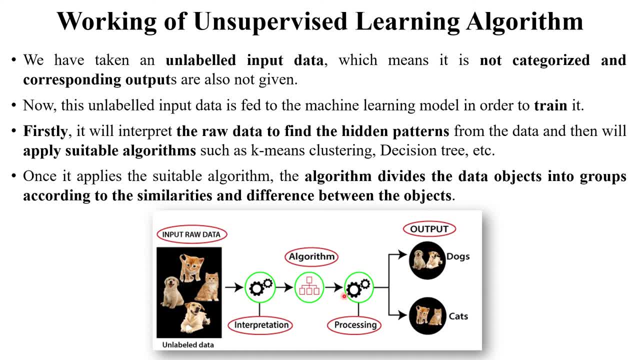 see, this is a working of unsupervised learning algorithm machine identify the patterns of those images and, as per their pattern, group the data. as per their characteristics. machine can be group the data or cluster the data by using some algorithms. so this is a working of unsupervised 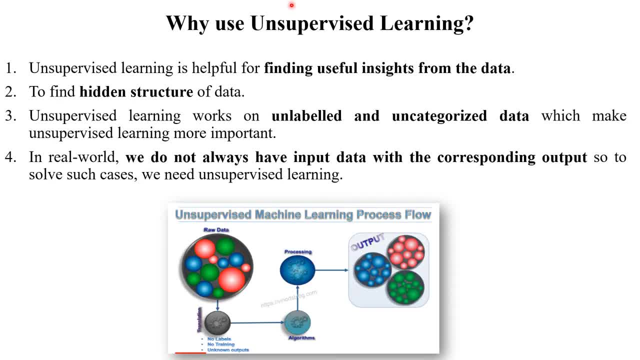 learning algorithms. next. now why we use unsupervised learning algorithm. so unsupervised learning algorithm is very helpful for finding the useful insights from the data. useful insights means some specification. unsupervised learning algorithm use different algorithms for find out the feature extraction, feature selection. this kind of approach purpose 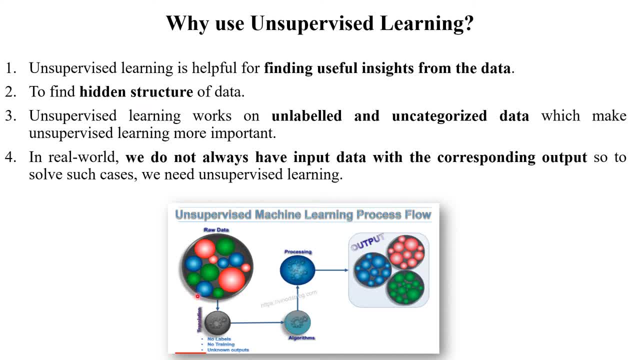 they find out the hidden structure of each and every data. right, they find out the structure of cat image and they find out the structure of dog image, so they find out the pattern of each and every image. this is a main use of unsupervised learning algorithm, then unsupervised learning. 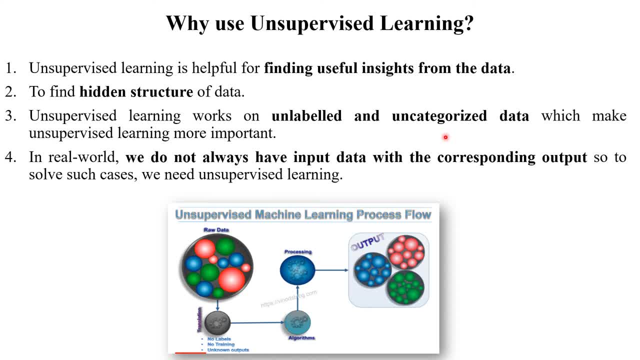 algorithm works on unlabeled data and uncategorized data. there is a combination of all kinds of data sets right so they can be grouped, those images, as per their features. in real world we do not always have an input data with corresponding output. right, nowadays there are large amount of data. 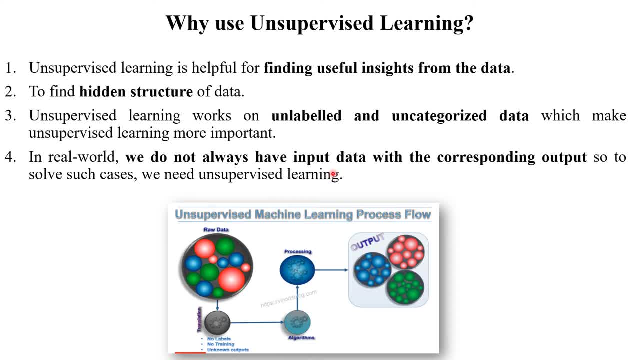 vast amount of data sets are available. sometimes data are in sorted format. sometimes data are not in sorted formats, so at the time, unsupervised learning algorithm is very useful for finding the useful to identifying the clustering of data set as per their similarities. so that's why we use 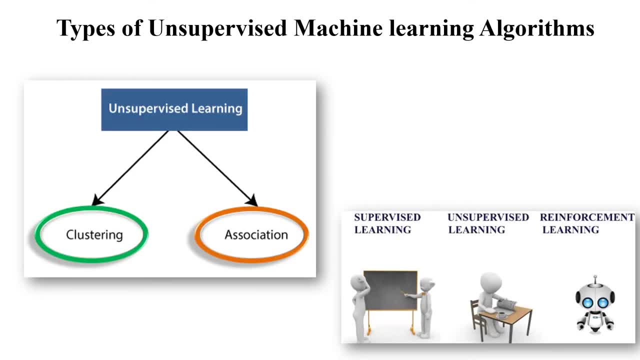 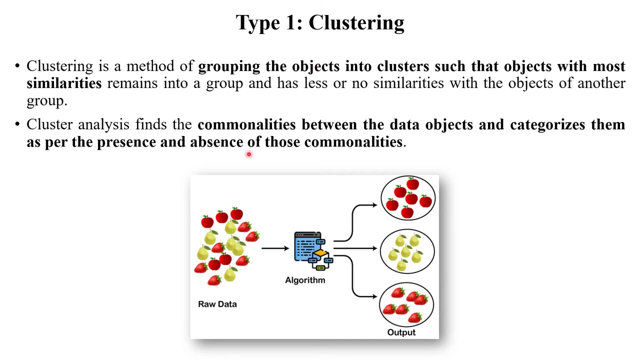 unsupervised learning algorithms. now, there are two types of unsupervised machine learning algorithms, that is, clustering and association. so let's see: the first type of unsupervised algorithm is clustering. so what is meant by clustering? so cluster, cluster means group, the group of similar. 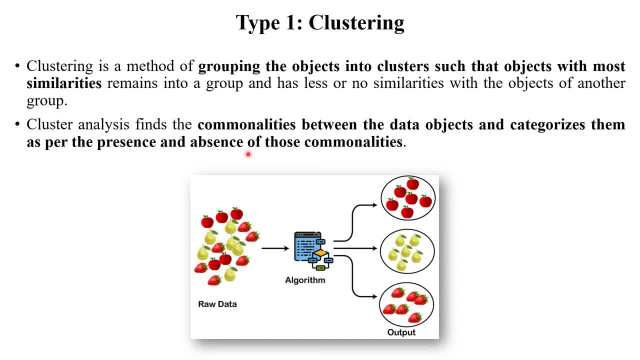 functionalities. this is called as cluster. okay, so clustering is a method to grouping the objects into the cluster which have been the most similarities. right, see in this diagram. suppose this is your raw data. okay, there are different images of strawberries and different images of apples and lemons, etc. so the particular machine identify the features, the patterns this particular 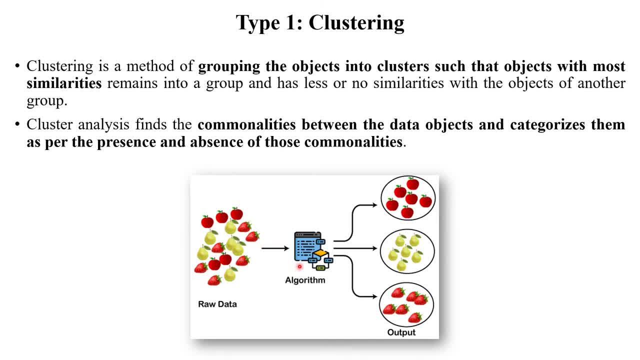 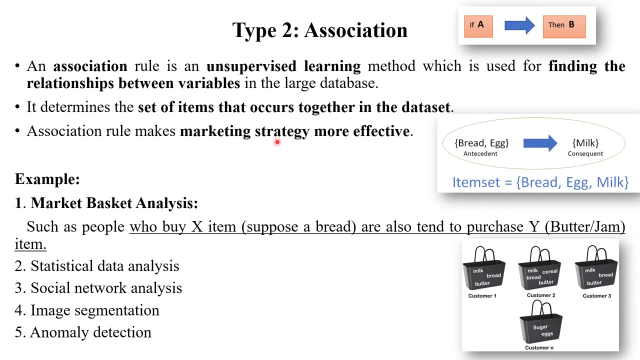 characteristics of that particular images and cluster those images as per their characteristics. this is a working of unsupervised learning algorithms. so cluster analysis finder commonalities between the data objects and categorize them as per the presence and absence of those commonalities. this is called as clustering. and now the next type of unsupervised algorithm is called as association. 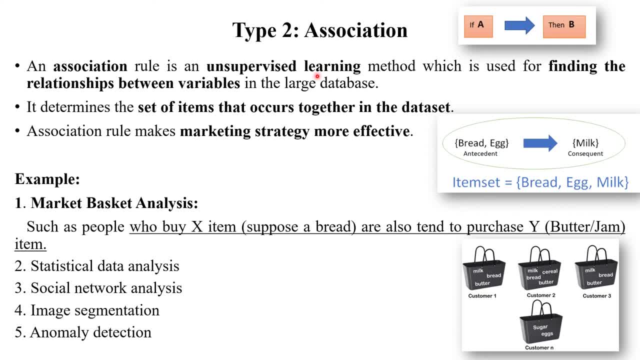 so association means to find out the relationship between the variables. the best example of association is the relationship between the variables, Market strategy or market basket analysis. Suppose a particular person buy X item, then they also buy a Y item. This is called as association. For example, see here: suppose a particular person buy a bread from supermarket, then they also buy a butter. So this is called as relation or relativity purpose of particular product. 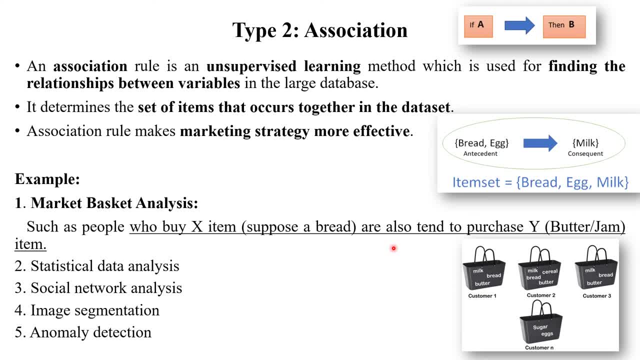 Suppose a particular customer buy a mobile, then they also buy a headphones, right? So analysis of all those data, or analysis of all those interrelated data, This is called as association. So it determine the set of items that occur and that can be purchased together. This is called as association. 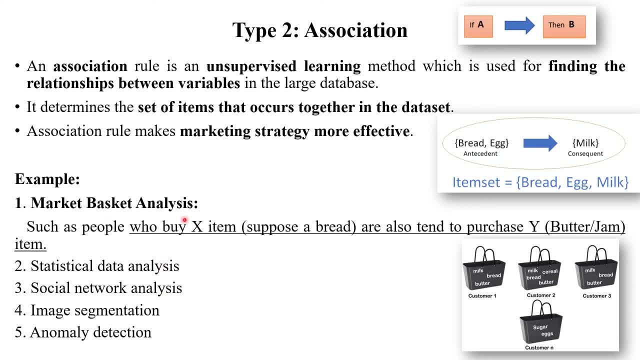 These are the different examples. that is, market basket analysis, then statistical data analysis, social network analysis, For example, Facebook. Facebook always gives you a suggestion regarding your nearest friend or the particular persons that working on same organization, same companies- right, It shows you a suggestion regarding this. It shows you a suggestion regarding friends, of friends, like this. So this is called as social network analysis, Then image segmentation, anomaly detection. So this is a concept of association And for that purpose we will use different unsupervised learning algorithms. 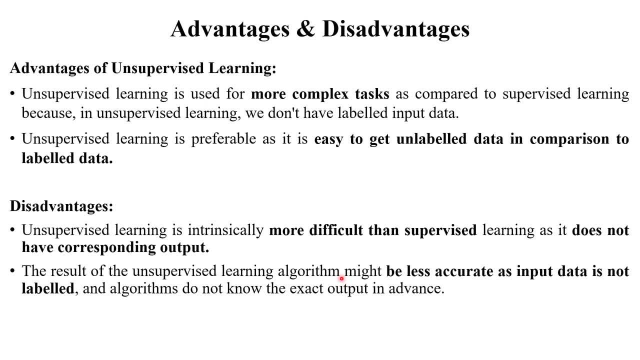 Now these are the some advantages and disadvantages of unsupervised learning algorithm. The advantages of unsupervised learning algorithms are: that will be useful for more complex tasks because it requires large amount of data sets. Labels are not necessary, right, So that will be used for more complex tasks. as compared to supervised learning algorithms, Then unsupervised learning algorithm preferable. It's very easy to get unlabeled data and comparison to label data, because nowadays it's very easy to get unlabeled data and comparison to label data.